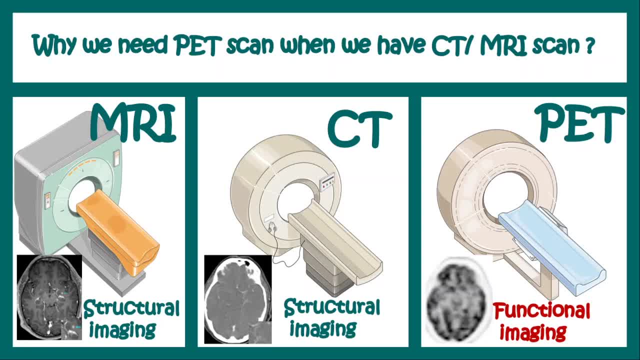 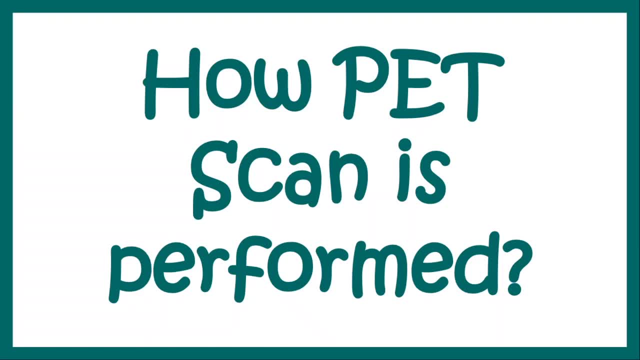 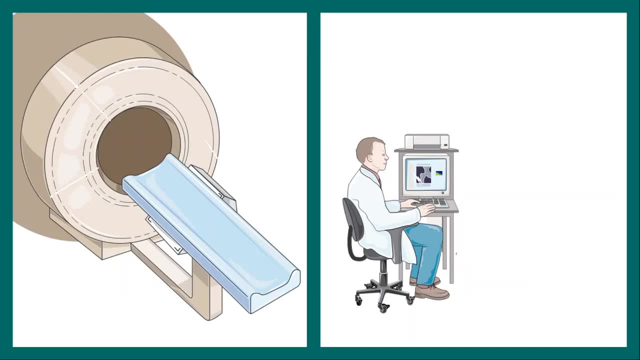 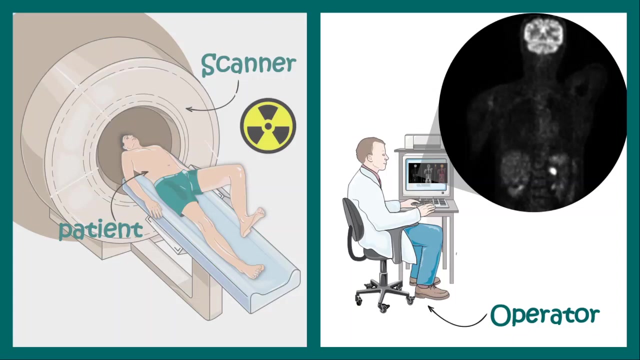 PET scan gives you a functional imaging. That means it shows the level of functioning or extent of functioning of those tissues. Now we will learn how PET scan is performed. Now the PET scan machine is kept in a separate radiation proof room. In the machine there's a scanner and in that machine the patient lies down and the patient is put into the machine tunnel. In a separate room the operator sits with a computer where the scan results are seen. Now, as I told you, this PET scan uses radiation and that's why this has to be kept in a radiation proof room. 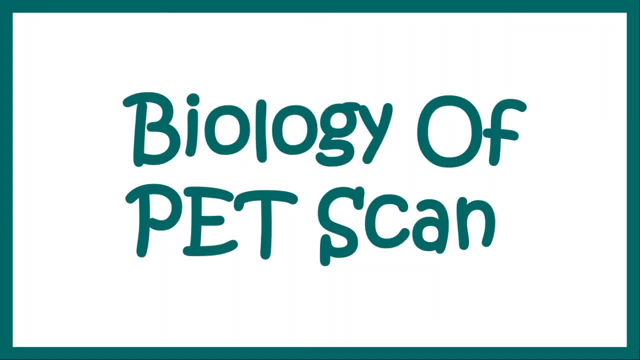 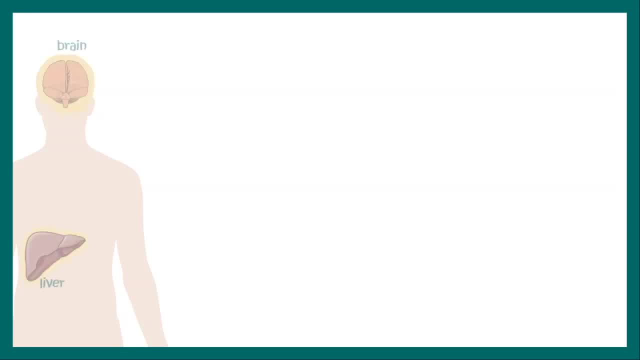 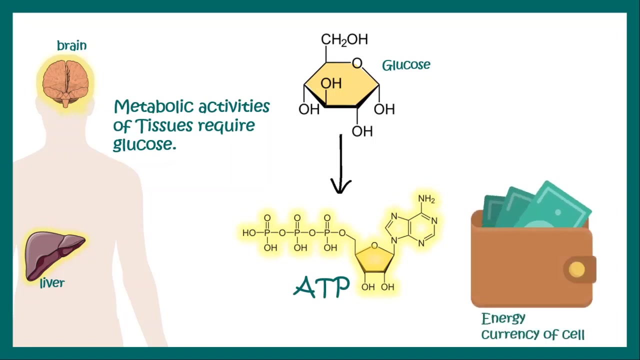 Now let us understand what biology plays behind the principles of PET scan. Now we all know that human body has different tissues, like brain and liver, whose metabolic activity requires glucose. Now glucose forms ATP by different metabolic pathways and this ATP is known as the Energy currency of the cell. This 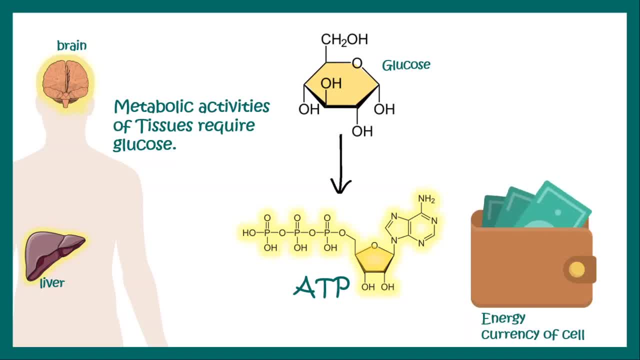 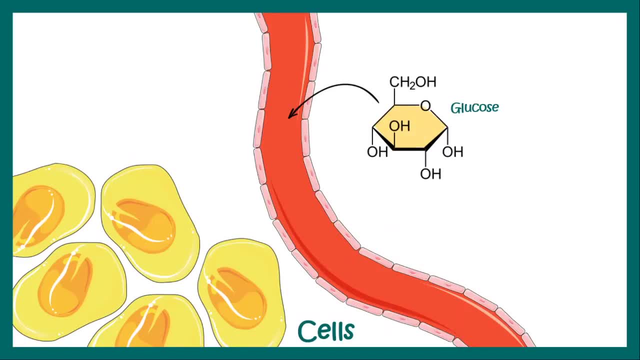 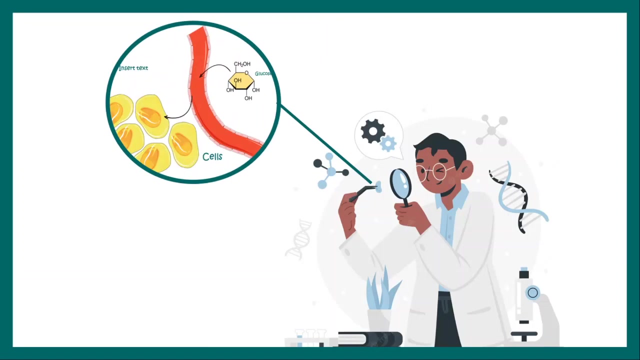 energy currency supplies, energy for different metabolic and cellular activity. house about pepper. pepper eaten, Dr CTOR, a mitre. Now this glucose is present in our bloodstream. whenever the cells require this glucose, they take up the glucose from the blood. Now this principle was exploited by the scientists to develop a scanning technique such as PET. 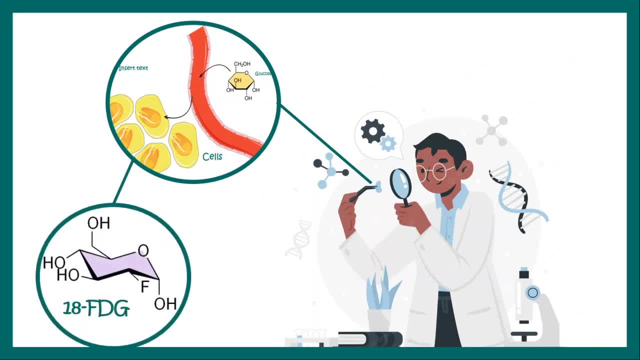 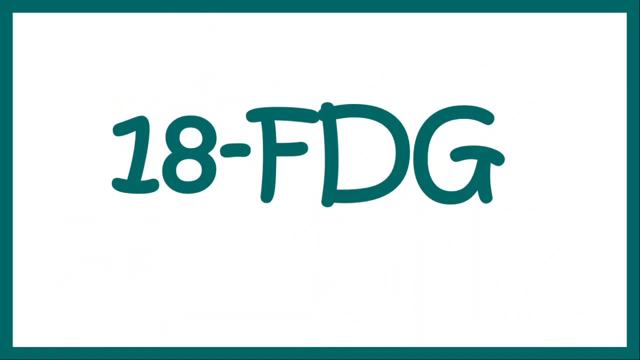 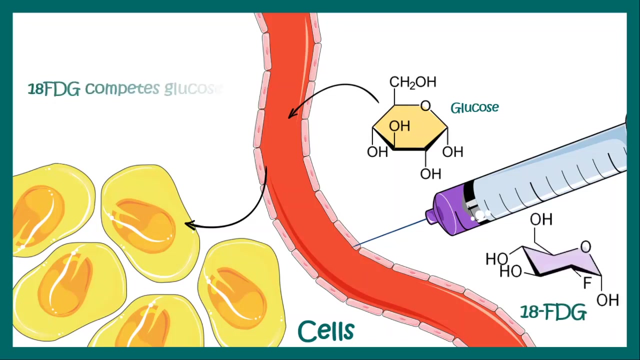 So they developed a molecule known as 18-FDG or 18-Fluorodeoxyglucose, which is a glucose analog which emits positrons, the antimatter analog of electron. Now let's learn more about 18-FDG Now. 18-FDG, when injected into the blood, competes with glucose for getting up taken in the cells. 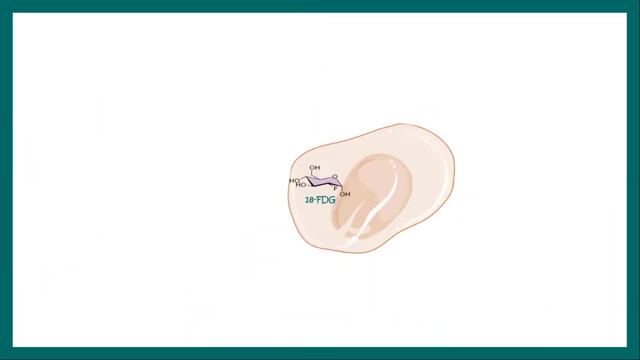 using similar mechanism. Now, when cells uptake the 18-FDG, 18-FDG emits positrons. Now these positrons come in contact with the electrons that are already present in different molecules of the cell, and electron is a matter. positron is the antimatter counterpart of. 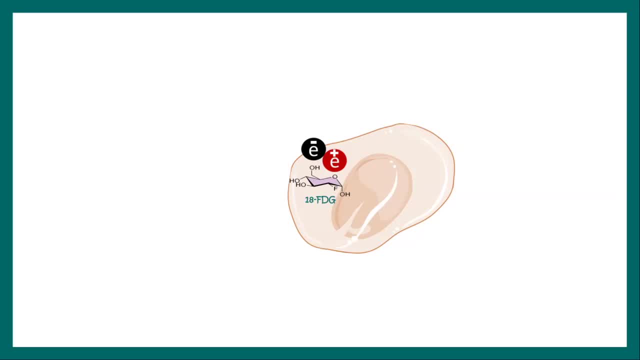 electron, So matter antimatter. when they come together in close contact, they undergo a reaction known as annihilation reaction. Now this annihilation reaction gives rise to gamma rays which go out in equal and opposite direction. These gamma rays are picked up by the scanner or the detector. 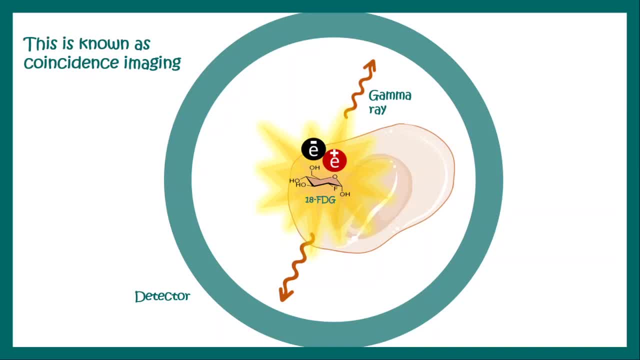 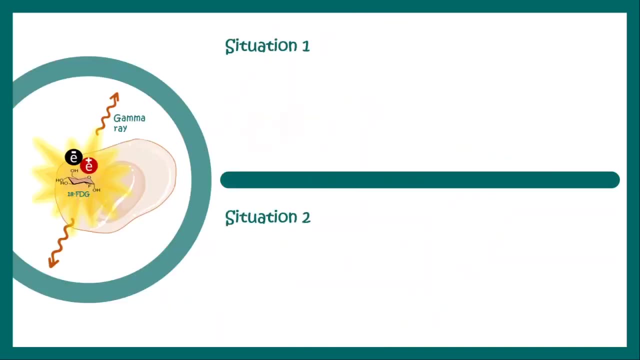 The two gamma rays moving in exactly opposite direction, picked up at the same point of time, is known as the coincidence imaging. So this is the core physics principle behind the PET scan. that is coincidence imaging. Now there can be two situations Now. in one situation, where we have highly metabolically active cells, they will take. 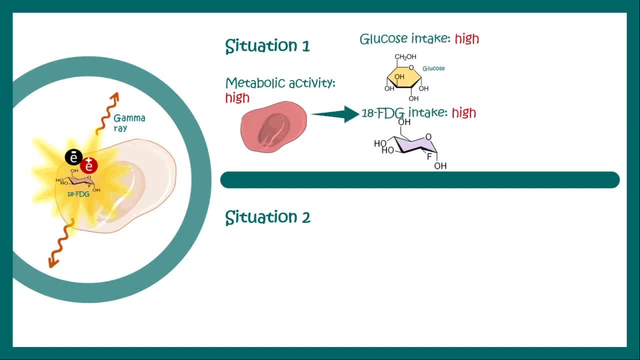 up a lot of glucose, and as they take up a lot of glucose, their FDG intake will also be high and hence they will emit a lot of gamma rays, because more amount of FDG will ensure more amount of annihilation reaction and from that we will get more amount of gamma. 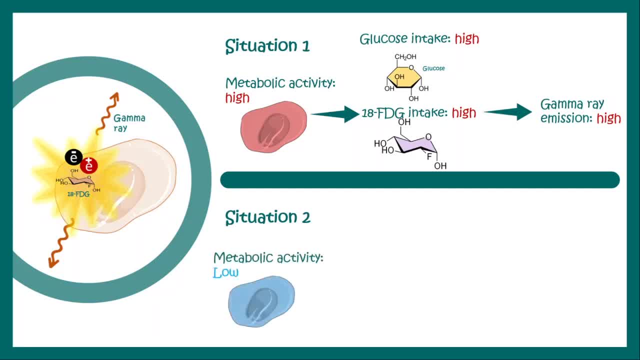 emission. On the other hand, in situation two, we have less metabolically active cells. they will take up less amount of glucose. similarly, they will take up less amount of FDG. less amount of FDG means less amount of positron. less amount of positron means less amount of annihilation. 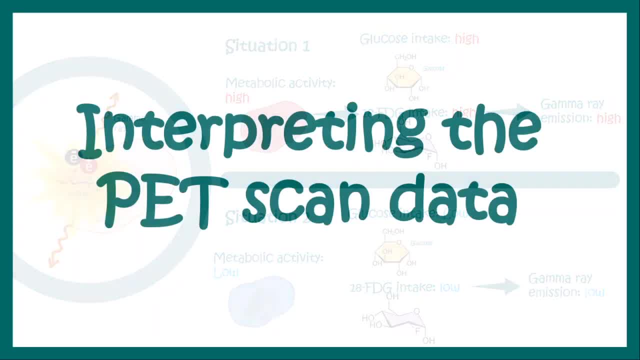 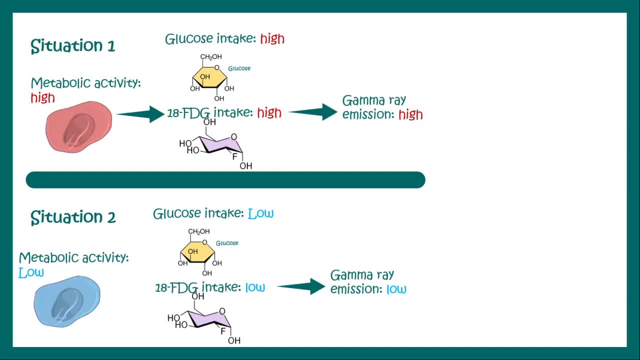 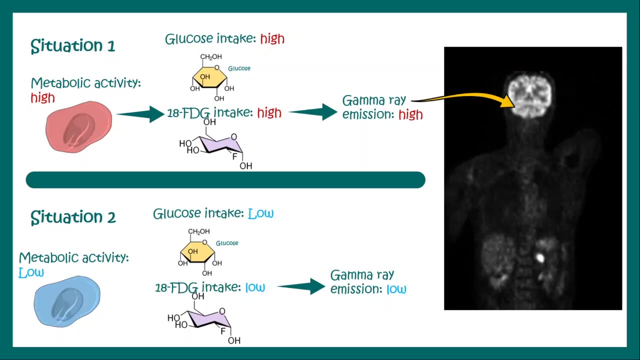 reaction, so gamma ray emission will be low. Now, based on these principles, let us interpret the PET scan data. Now, in situation one where we have gamma emission high, we can see in the image that will give you a high or dense signal. This is known as a hot spot. 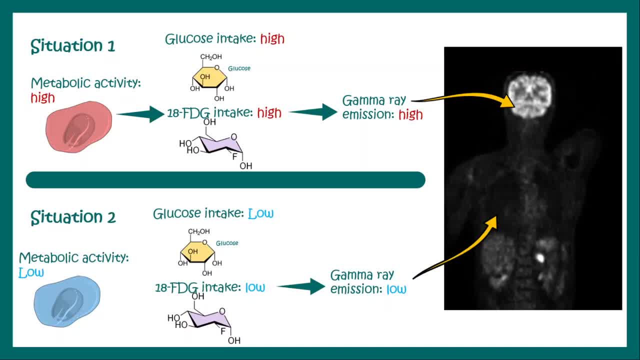 Whereas when metabolic activity is low, gamma emission is low. that gives rise to a low signal, or low density signal, known as a cold spot. This hot spot and cold spot gives you an idea of differentiation. So this is the cold spot. Okay, So 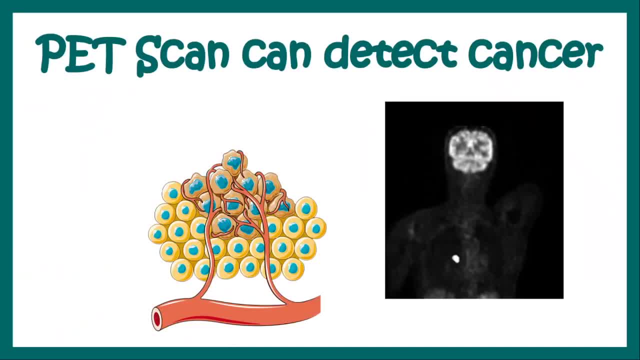 Okay, So, So, So, So So level of metabolic activity in different tissue. now this PET scan can also detect cancer. like cancer, cells are glucose hungry cells because they have a high level of metabolism as well as very much increased cellular activity. say, as they take up lot amount of glucose, they also take up a 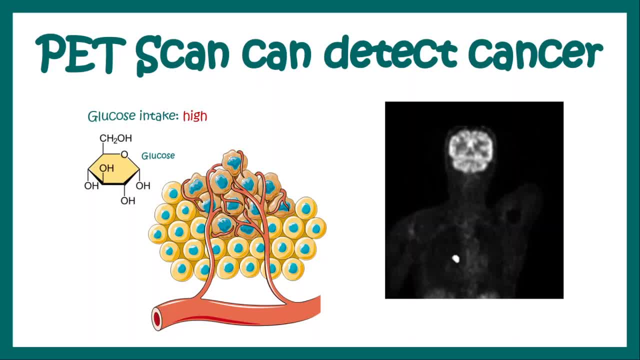 lot amount of 18 FDG and hence they give high density gamma emissions or a hot spot, as you can see in the image of this PET scan. but, my friend, the problem is not over yet. you can see a hot spot near the lungs in the thorax, but, but from this image you cannot actually tell whether the hot 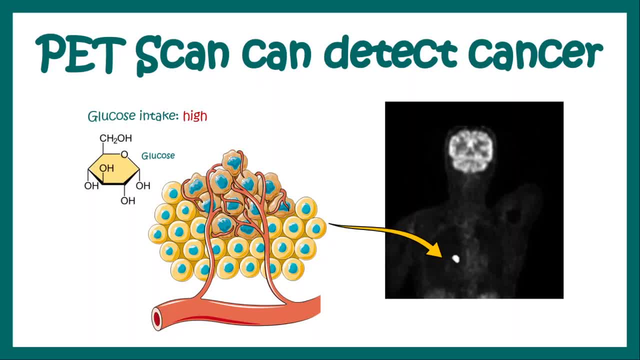 spot is in the lungs or in the heart or in some mediastinal organ, because the quality of this image or the resolution of this image is quite low and based on this imaging only. a doctor cannot comment on the particular location of the tumor you can see in the image of this PET scan. but, my friend, the problem is not over yet. you can see a. 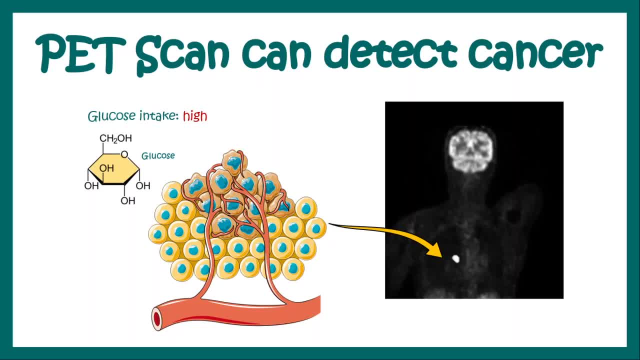 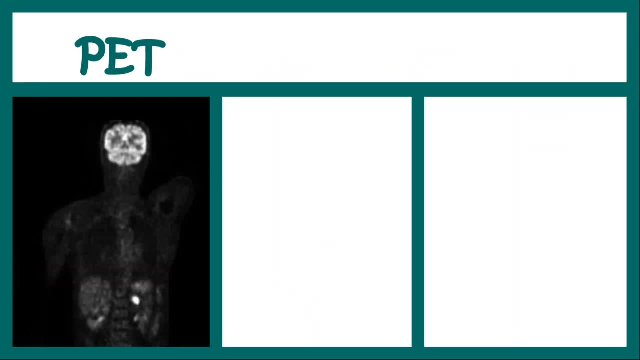 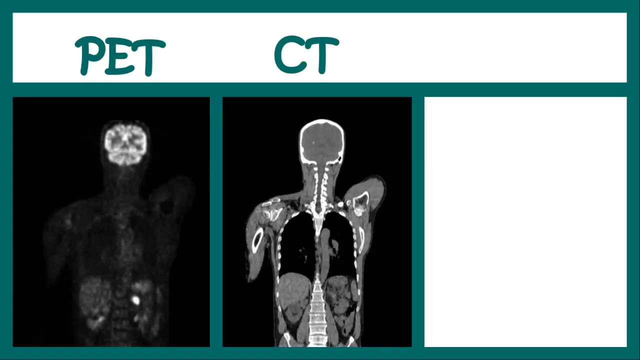 cancer, so a doctor needs more. so here the scientists again brought about a change. that means they took the PET scan. similarly, they took a CT scan. now CT scan is known, or MRI scan is known, for their high resolution images and they give you higher level of anatomical or structural 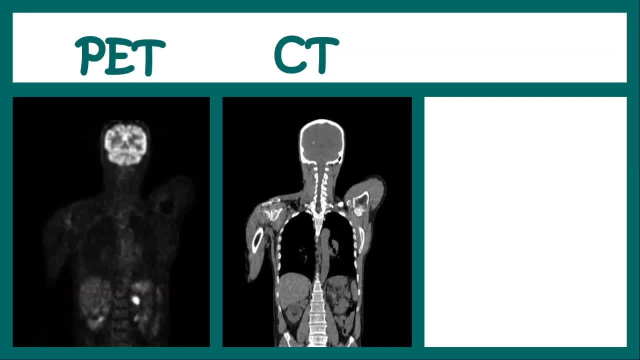 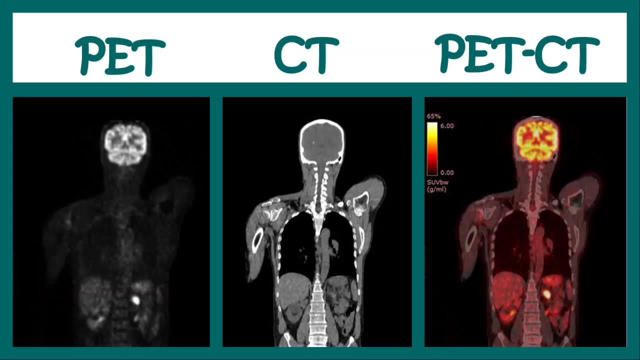 localization. now, using proper softwares, they superimpose these two images to get something known as a PET CT. Here you get the metabolic activity along with the anatomical localization of that particular metabolic activity. so in that way you can find out a highly metabolic spot or a hot spot. and 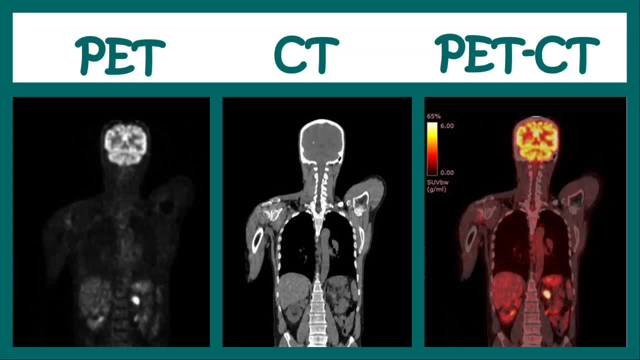 also, you can know exactly in which anatomical structure or in which anatomical location your particular hot spot lies. that that gives you an opportunity to localize the lesion in a particular way. so, in summary what we learned? we learned that PET scan technique is very important for the 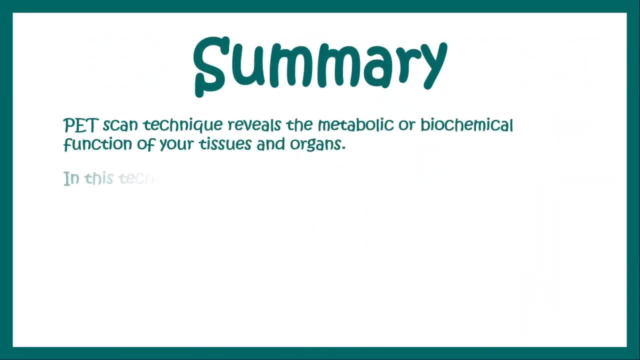 detection of cancer and it reveals the metabolic or biochemical functioning of your tissues and organs. in this technique, the key player is the positron, which is the antimatter counterpart of electron, and the gamma ray emission, which is picked up by the detector by coincidence imaging. the mechanism of PET scan: we learned in detail the annihilation reaction, coincidence imaging, gamma ray emission, etc. and finally we learned that PET scan can be used to detect metabolically active lesions such as cancer. now we also learned how to 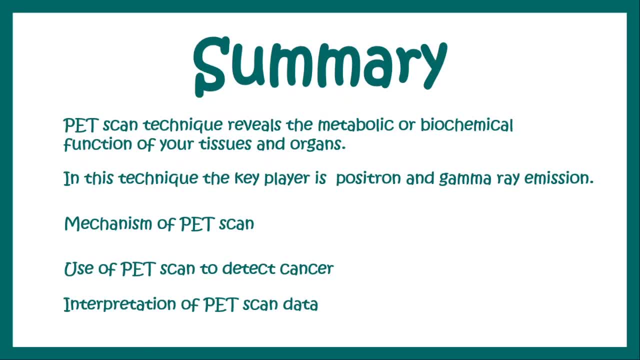 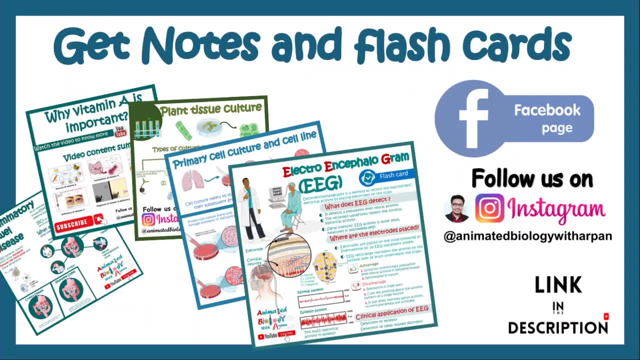 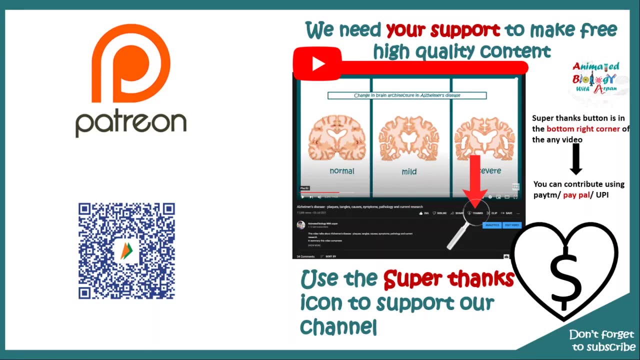 interpret the PET scan data based on the two scenarios that we took up beyond: hot spot and cold spots. now to get notes and flash cards, you can follow the facebook page and instagram of animated biologies with arpan. the link will be in the description. also, you can support this channel so that we can keep on making high quality content on patreon. also, you can go for a super thanks by clicking on the super thanks button on the bottom right corner of the video and you can contribute using